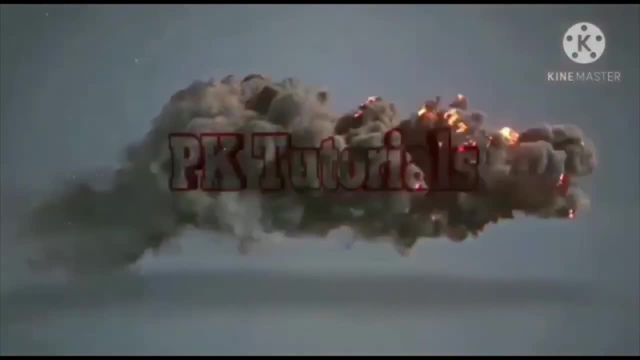 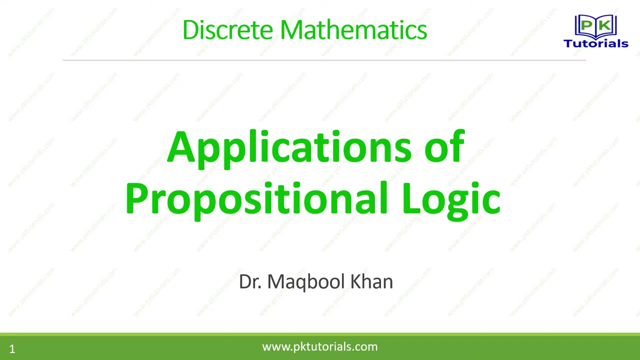 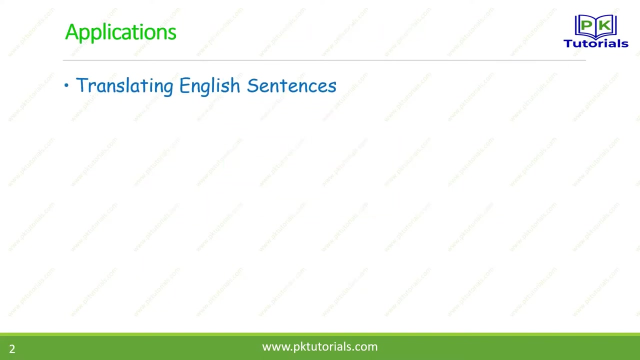 hello, welcome to pktutorialcom. so today our topic is about applications of prepositional logic, so let's begin. so the first application that we will discuss is translating English sentences. English sentence: ko hum prepositional logic mein keistara convert kar sakte hai, ya translate kar sakte hai. second, hai boolean searches. 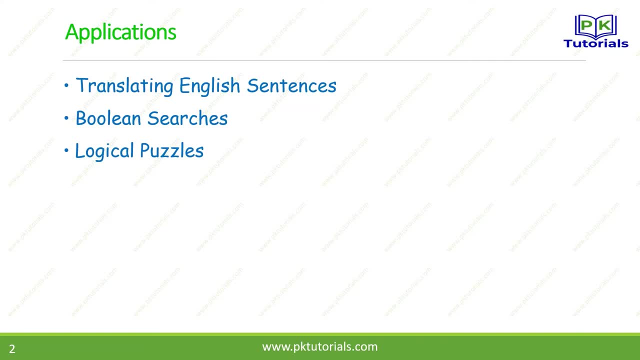 aur third hai logical puzzles, aur chota hai logical circuits. so iss current lecture mein hum first three ko dekhte hai, logical circuit, ko next video mein cover karte hai. so first hum dekhte hain steps ko, ki humne kitne step mein English sentence ko translate: 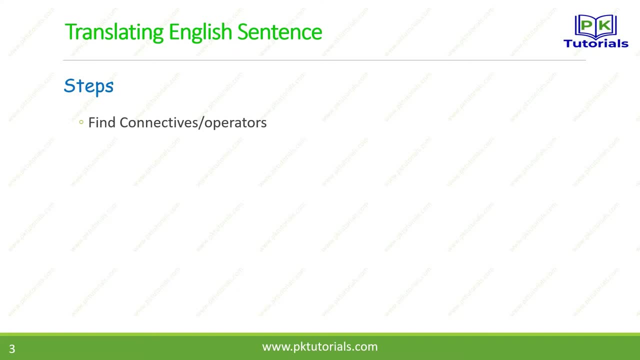 karna hai. first step hai humare paas find connectives or operator. jo connectives hai, jo sentence ko milate hain, apas mein hum usko search karte hain given sentence mein. secondly, jo long sentence hota hai, usko humne break karna hai aur rename karna hai short sentence. 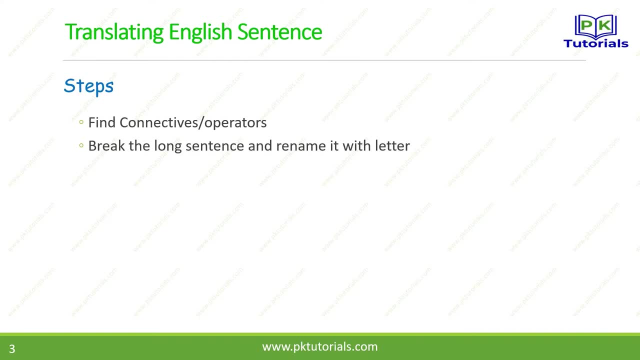 ko with some letter like p, q, r, any letter that you want, aur iss ke baad humne construct karna hai preposition ko. so let's have a look at some examples. example hain humare paas. to take discrete mathematics, you must have taken calculus. 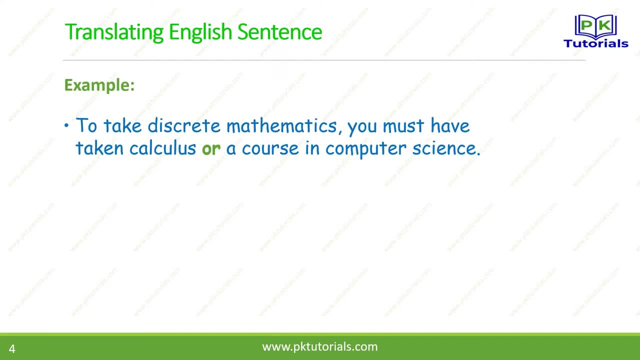 or a course in computer science. yaini discrete mathematics ki course lene ke liye aapne pehle se calculus para ho. yaa kui bhi computer science ka course liya ho, pir aap usko le sakte haiso. 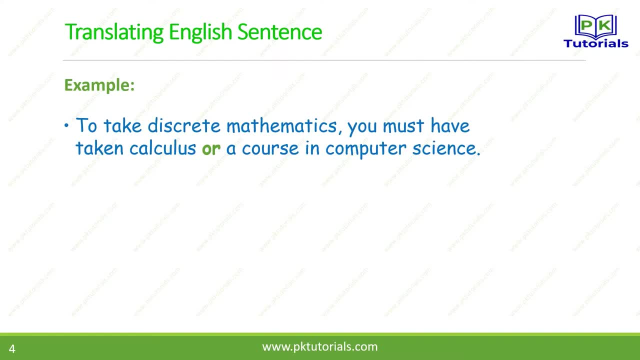 iss ko hum convert karte karte hain prepositional logic mein. so jo step tha humare paas ke humne logical isme connectives doon na hai find to connective. humare paas r hai ek to means ke r ke baad. 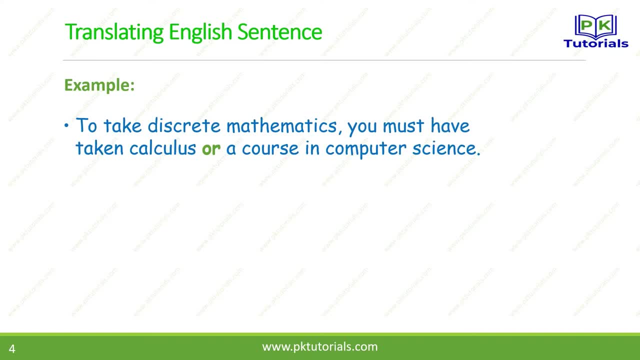 jo sentence hai, iss ko hum break kar sakte hain. issi tara, jo first sentence hain, part j. to take discrete mathematics, jo comma hain, uske bhi hum break kar sakte hain. to we can assign letters, aur iss ko hum assign karte hain letter se taa ki short form mein. 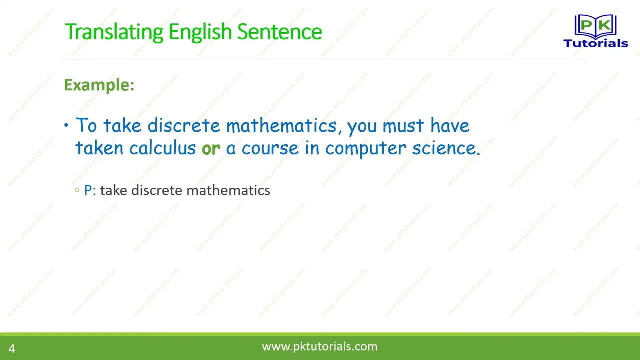 aa jaye. so let's suppose that we represent. take discrete mathematics by p, hum isko p se denote karte hain. issi tara to take calculus denoted by q, aur issi tara take course in computer science. we assign r letter, so kui bhi letter aap assign kar sakte, zoroori nahin ke p kyun r ho. 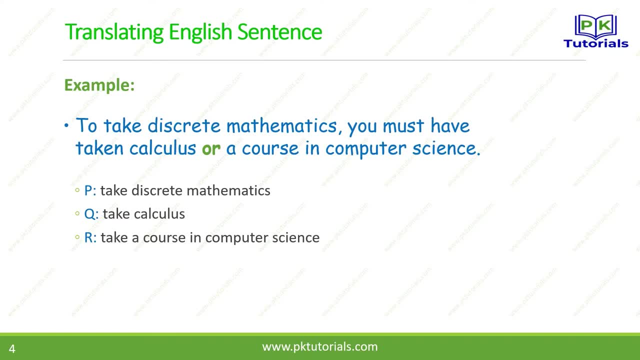 to jo third step tha, ki humne aap se construct karna hai, propositionab dekhe, jo connective hain r ye humare paas equal tha. iss ko hum disjunction kehte hain. yaini in doonon mein se take calculus or course in computer science kui bhi ek, jab kui bhi ek ho to disjunction. 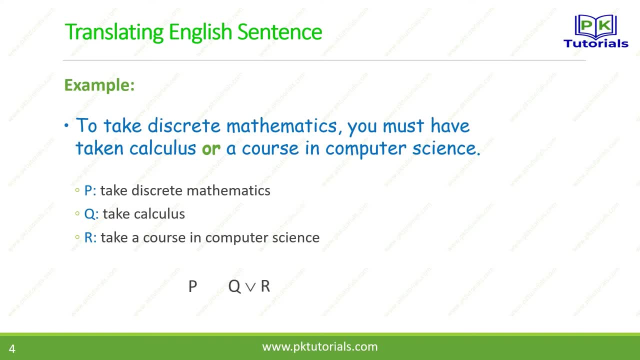 se hum iss ko represent kar se dekhe, se dekhe, kyun disjunction r yaini in doonon mein se kui ab jo first hain to take discrete mathematics. ye ek condition hain, aur iss condition kyun hum kiss se denote karte hain. 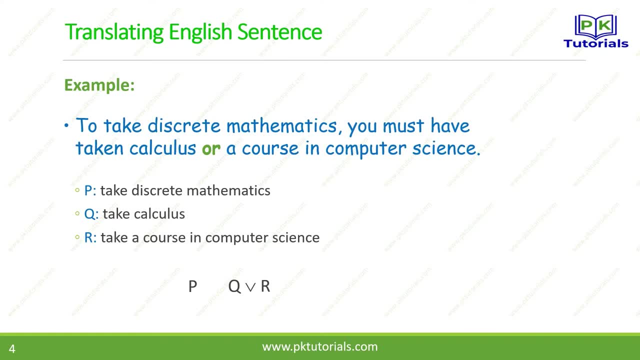 humne last pehle lecture mein padha tha: implication: ye sign tha uska ki p implies that kyun disjunction r yaini discrete mathematics course lene ke liye. aapne calculus ya course in computer science doonon mein se ek lene chahiye. 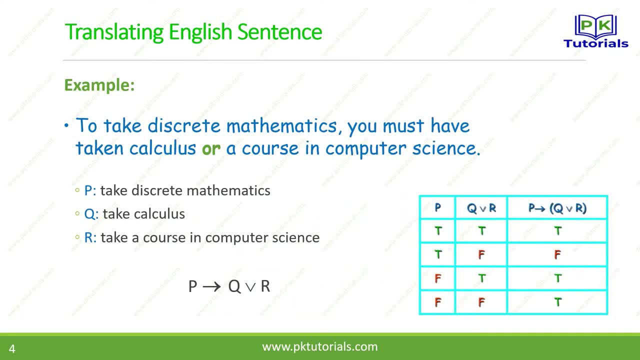 iss ko hum truth table se bhi denote kar sakte hain to p hain a value, possible value. hum check kar sakte truth value, se ki p ke possible value ke tne hai, true, true. and issi tara jo kyun disjunction r hai, uski bhi hum draw kar sakte to purik. 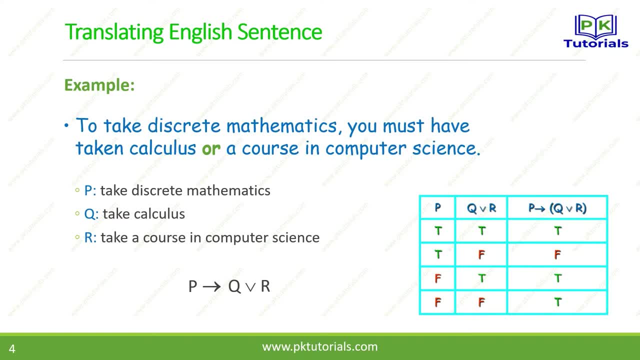 mein hum kitne possibility ho sakte, agar p humare paas true ho. yaini discrete mathematics liye ho to kyun jo taken course in calculus or course in computer science. yaini doonon mein course se liye ho to means, ki kyun disjunction r bhi true hoga. 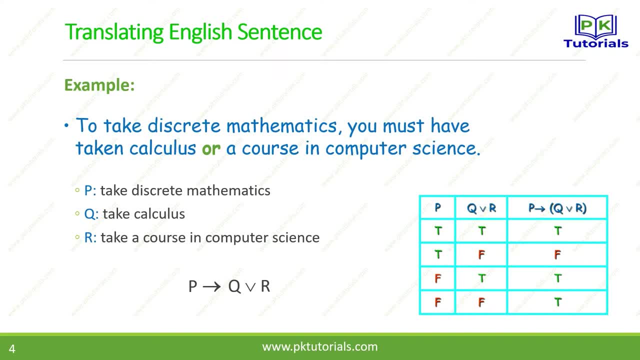 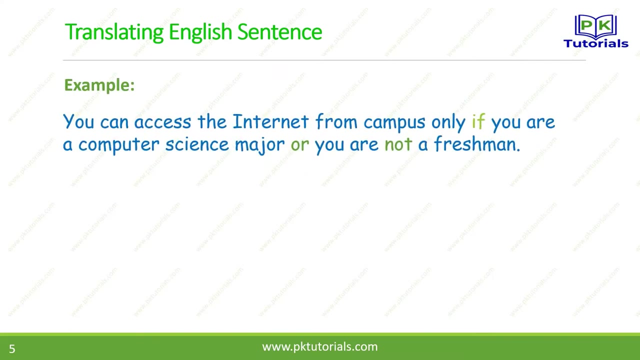 to p hain to ye implication humare paas true ho sakte hai. so you can check all this truth table for to verify the condition aaye dekhte hain ek dusra example. example hain humare paas. you can access the internet from campus only if you are a computer science major or you. 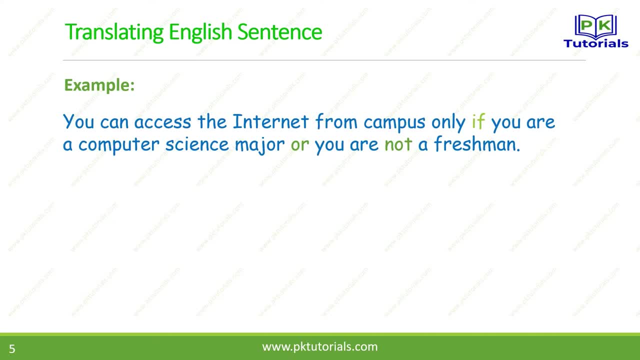 are not a freshman. bada simple hain. agar internet access karna ho, toh aap computer science major ke student ho, ya aap koi freshman nahi ho, toh first jo step tha, ke humne koi connect you doonna hai. connect you, isme R hai, NOT bhi hai. 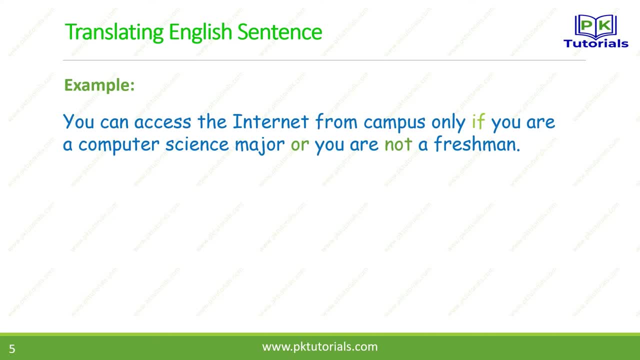 aur issi tara jo sentence ko hum break kar sakte, if ke baad bhi hum break kar sakte hai. so let's break the sentence and the first part. you can access the internet from campus, isko hum aise represent karte hai. issi tara, you are a computer science major, isko hum C se denote karte hai. aur. 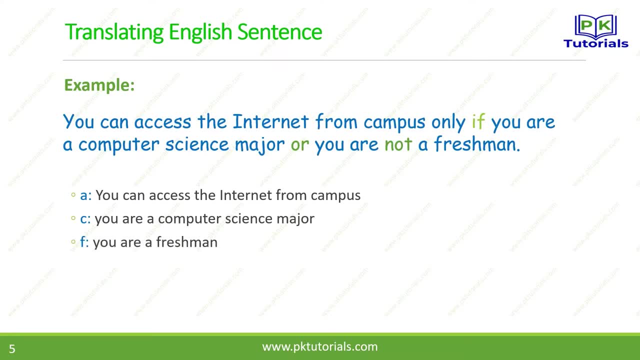 third hai you are a freshman. if toh idhar jo humara ek hai negation. NOT toh jo if hoga humare pass un negation. if ho aega you are not a freshman, toh iss ka jo preposition banda hai C ko jis tera last example me humne disjunction liya tha C aur F. 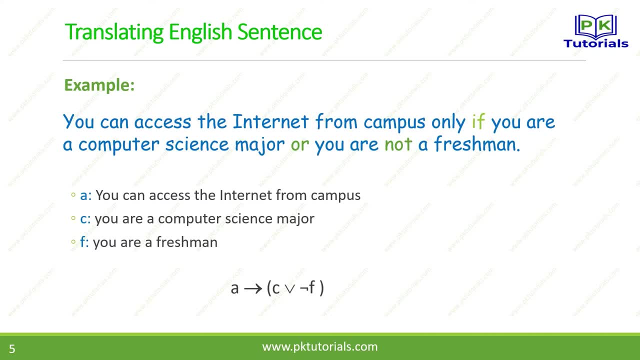 F kar leken hum idhar negation of F. yaini, you are not a freshman. you are a freshman is F and you are not a freshman. negation of F. toh ain doonun ke jo condition hai ke oh hum implications ke stroh. 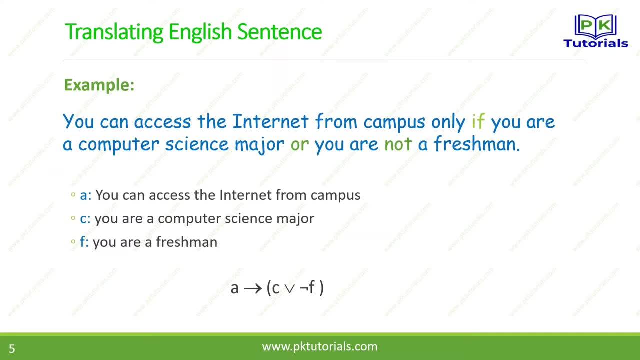 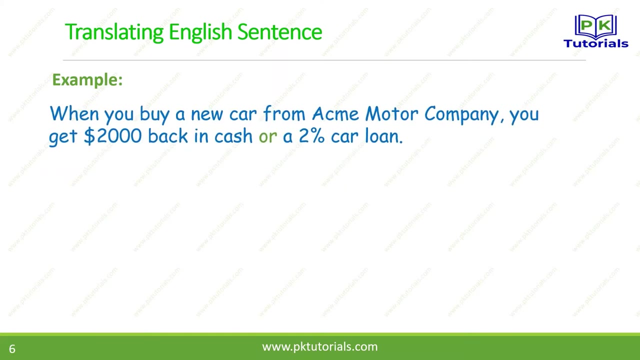 zahir kar sakte hai. so A implies that C disjunction negation of F, yeh isska preposition baniga iss sentence ka. let's have to look another example. example hun mere pass: when you buy a new car from Acme motor company, you get $2,000 Drawback. Genge are a 2% car Loan. 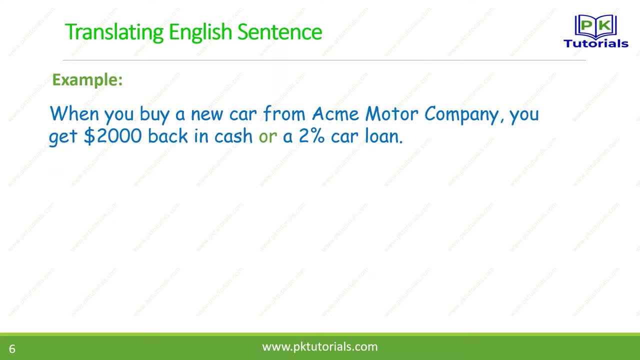 es hi inquiry, he sock jo r hai. yeh humare paas connect you hai, aur iske baad hum letter assign karte hai. so lets p represent: buy a car from acme motor. buy karna hai humne car acme motor se acha jo. 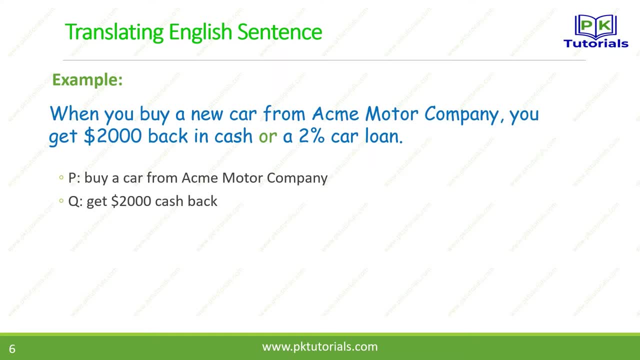 discount hai. o deray, get $2000 cash back. represent it by q aur issi tara r se hum represent karte. get a 2% car loan. acha, issme thoda sa logic hai, ke issko humne preposition banana hai. 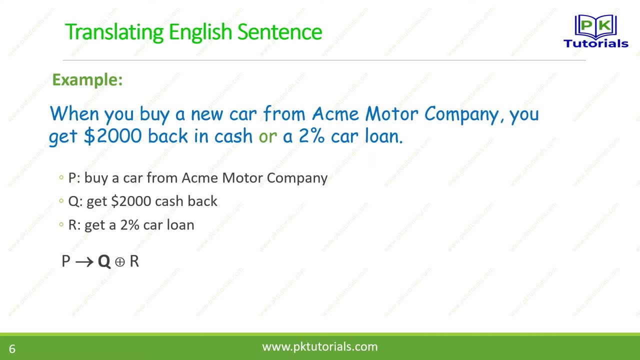 issme humne exclusive r use karna hai. p implies, that kyun exclusive r kyun use karna hai, because when r is used in its exclusive sense, the statement p or kyun means p or kyun, but not both. dekhe yeh jo company ne offer diya hai, motor car purchase karne ke ban yeh aap. 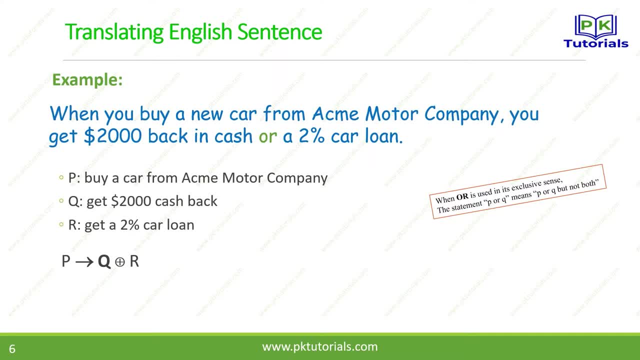 kyun ya $2000 denge ya 2% car lenge ya dono nahi de sakte hai, but not both means p or kyun, not both. agar hum both ka option available ho to aur disjunction function mein hai, jo humne last example mein kiya r disjunction operator to usko hum use kar sakte hai, but 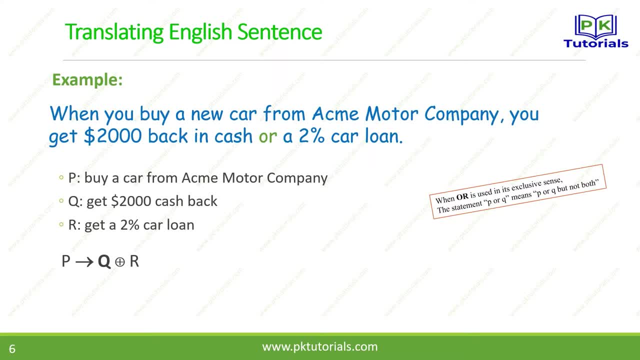 agar dono ko at a time aap avail nahi kar sakte hai, pir humne exclusive r ko use karna hai. is baat ka dyan rakhe ki humne koonsa r, jab bhi r ata hai ki us karna hai. ya simple r. 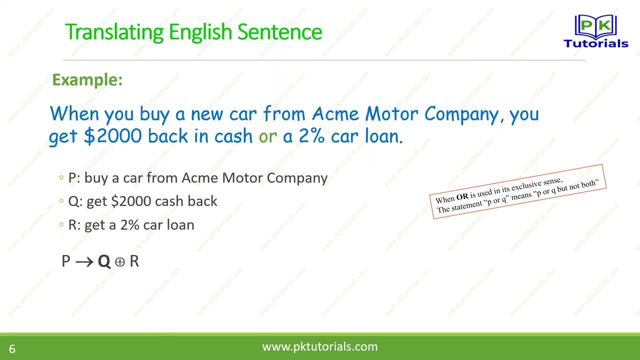 use karna hai disjunction to iss exclusive r ko todhasa jab bi use karna ho, isske liya todhasa fakar karna jaiye is ka jo truth table hai. yeh deke kyun aur r agar humare paas simple. 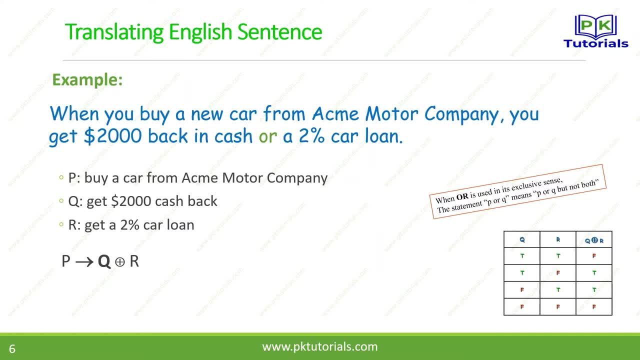 junction function hota to edge your last option. first option hota jab do no true who to either true, I am a capacity like in either Hamaripas, false IAQ, don't know. your discount offer, hey, oh, don't wait a time. well, no, second. so 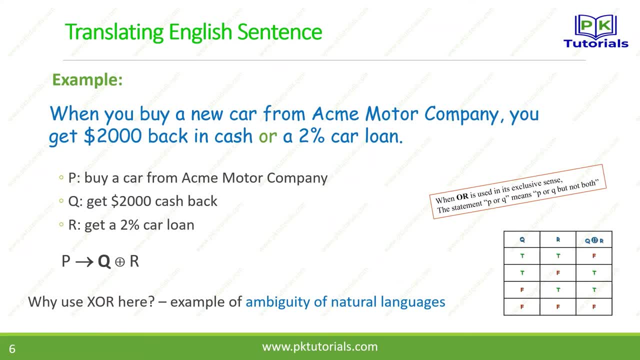 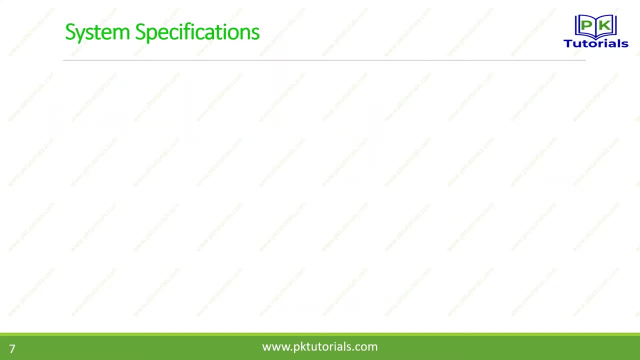 that's where the exam we use exclusive are here, because example of ambiguity of natural languages, or each example, homily, I am big witty of natural language, cookies me ambiguity, the argument discuss, captain, big witty, chaotic. system specification. system specification, jota, hey, okay, Hamlet is a system. could banana head to us comedy palace specify Karna? 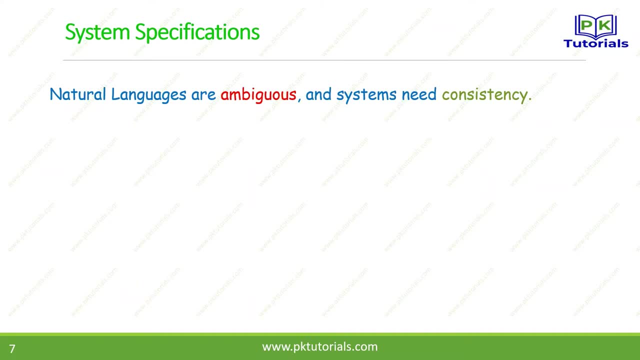 hey to. natural languages are ambiguous and systems need consistency. nature is to Hamar. English language history: you, you, I'm big- was a or just system. Hamlet design Karna a computer base. pay us cook consistency, dark are ODM. just our Hamlet. previous example made a cocky. 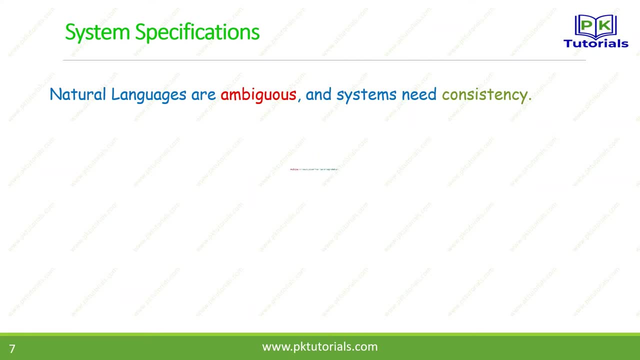 Hamlet are use Karna, exclusive are. so you're a ambiguity. ambiguity means having more than one interpretation of your art. a Hamaripas previous example: me English, me what he are you. so that was my exclusive are, co-option, a key exclusive are. hey, yes, simple disjunction. 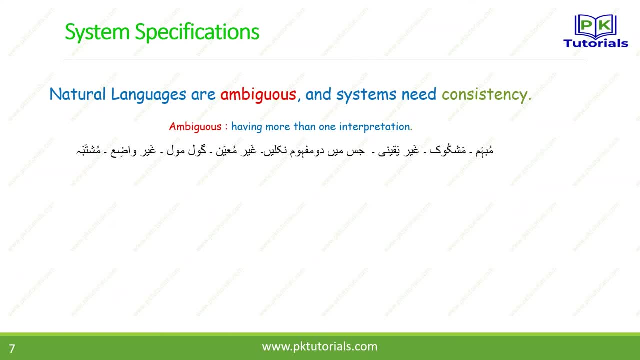 are a key agar money, dickage a. or do me to ambiguous means, move him Musko grater. he neither both sarala fuzzy or the a just me doom of form. Nick Levera, Hermione cool mole, rare was a much tab a to English kibbutz are a word may have. 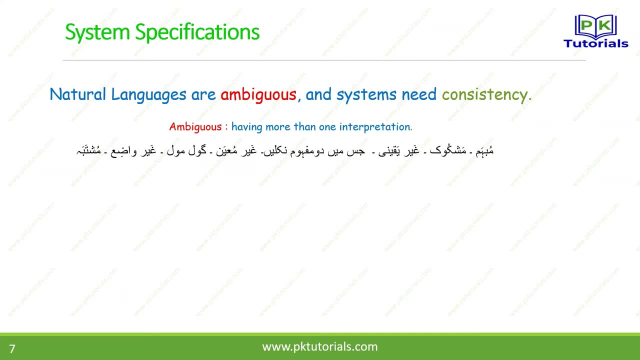 just me in big witty or tea stir acacia, do my form with a key to get in with a keeshamy. Shubha Kushti, Amrita Shubha. Shubha Kushti, Amrita Kushti, Amrita Shubha. 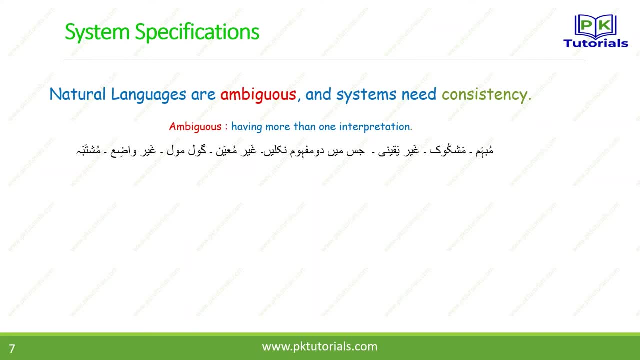 It is ambiguous. it is an illusion or it is not clear, or there are different types of ambiguities in it, So it is called ambiguous. So natural languages are ambiguous and systems need consistencies. What is consistency? Consistency means they should not contain conflicting requirements that could be used to derive contradiction. 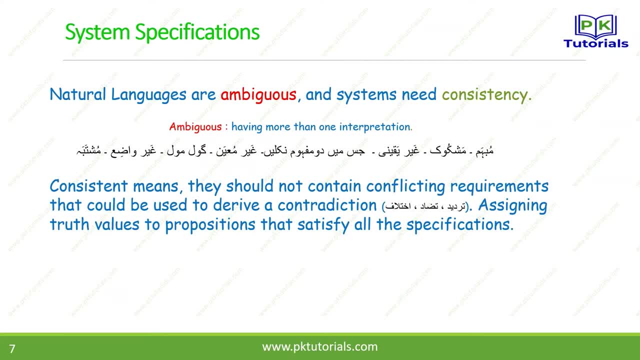 Means. contradiction is assigning truth values to propositions that satisfy all the specifications. All the specifications are assigned to the propositions that satisfy all the specifications. Consistency means consistent, consistent, consistent, consistent, So consistent when specifications are not consistent, If the specifications are not consistent, there would be no way to develop a system that satisfies all the specifications. 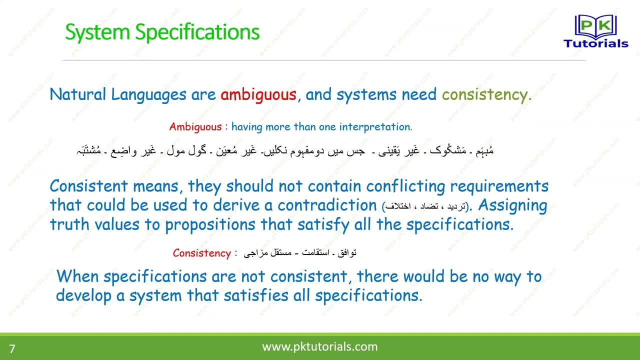 So the system that we develop for the machine, the system which we develop for the machine, we will not be able to satisfy all the specifications. that's why we need to remove ambiguity. so the biggest benefit of this is that we remove the ambiguity of natural language. 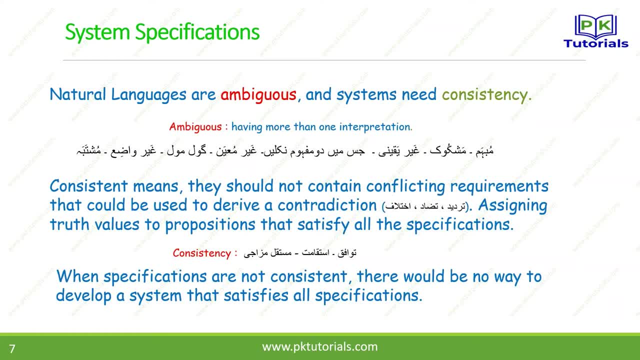 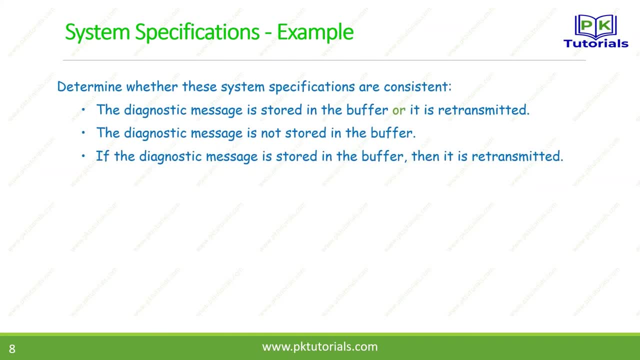 and we make consistent system. let's see an example of system specification. we have the example determine whether this system specification are consistent. we have given three sentences to check whether this specification is consistent or not. first sentence is: the diagnostic message is stored in the buffer R. 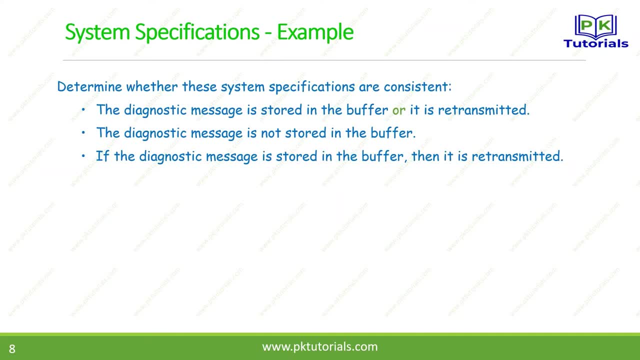 it is retransmitted. R is connected to us, so we can break this sentence here. the diagnostic message is not stored in the buffer. this first part is the negation of that, which is the first part of the first sentence. if the diagnostic message is not stored in the buffer, 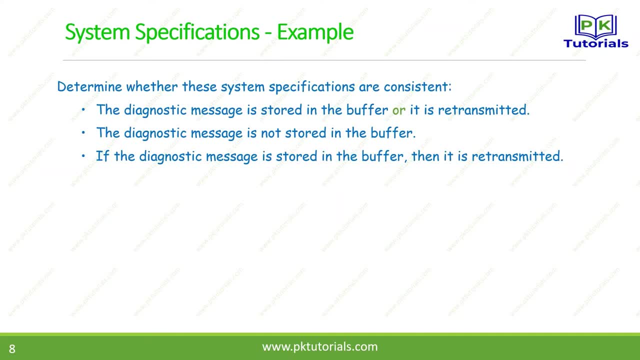 then it is retransmitted. so you can ask for the third sentence from these two. if we denote it with a letter, let's denote the diagnostic message stored in the buffer. the second sentence is why the diagnostic message is retransmitted. we can represent these three lines: 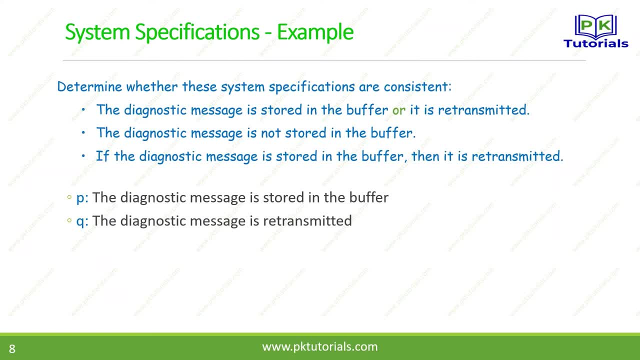 with these two suppositions. the first sentence is why we have P disjunction. we have used the disjunction of R, that why P is R. the message is stored in the buffer R. it is retransmitted, so we can denote P disjunction Q. the second sentence is the simple negation of P. 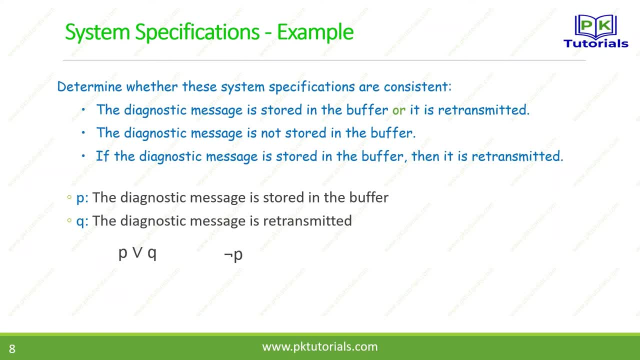 the first part of P. the diagnostic message is not stored in the buffer, so we can represent it with the negation of P. the third sentence is the implication, because when the condition of if-then comes, we can mostly use the implication if the diagnostic message is stored in the buffer. 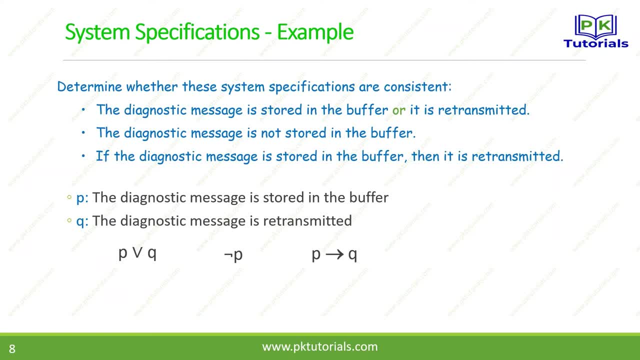 if the diagnostic message is stored in the buffer, then it means that it has been retransmitted. so P implies that Q. we had read the implication in the last lecture. so these specifications are consistent because they are all true. when P is false and Q is true. 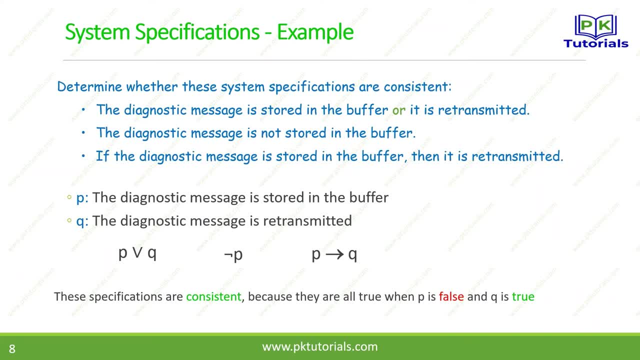 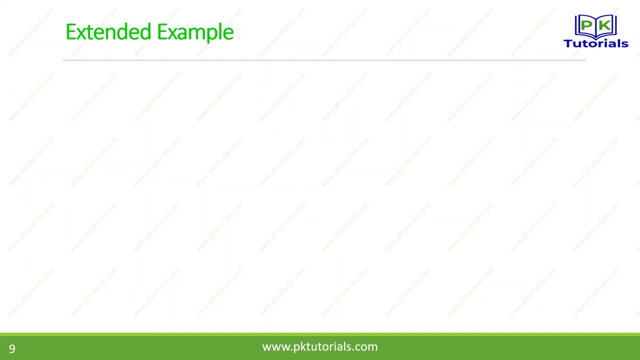 if P is false and Q is true, then all these specifications are true. there is no ambiguity. there is no ambiguity. there is no logical flaws in it. so we call these specifications are consistent. we extend the same example so that we can see the non-consistency. the fourth line of the first example is: 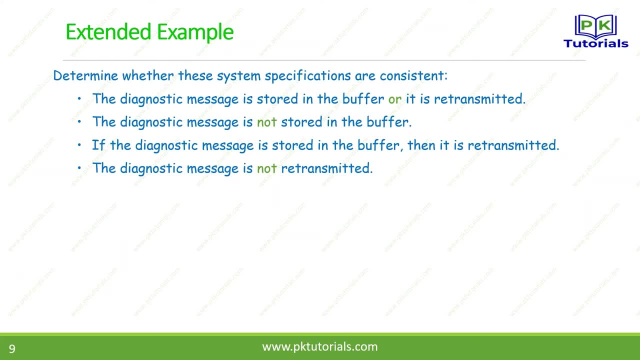 the diagnostic message is not retransmitted. ok, so this is the specification of the system. so let's check it. the supposition is the same as in the last example of P and Q. now this P, which we had done in the last of the three sentences. 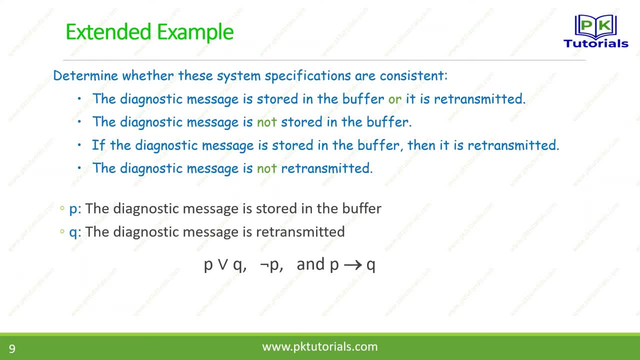 is the same as P. disjunction of Q. negation of P and P implies that Q. but if we look here, negation of Q is false when Q is true. if we have Q, true means the diagnostic message is retransmitted. if this retransmitted sentence is true, 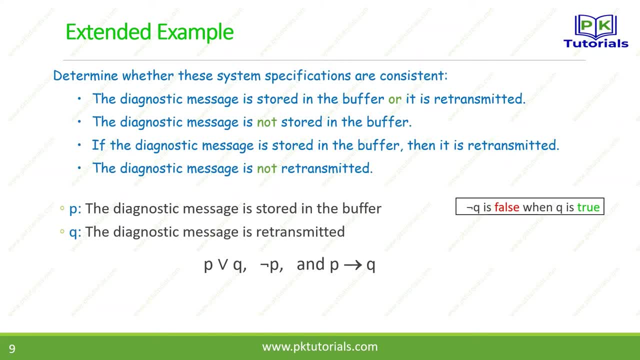 then negation of Q is false. so we have false, which is the fourth sentence. we cannot follow it because the diagnostic is not retransmitted. it means that there is ambiguity, because these sentences, this fourth sentence, it collides with it, it contradicts with the first implication. 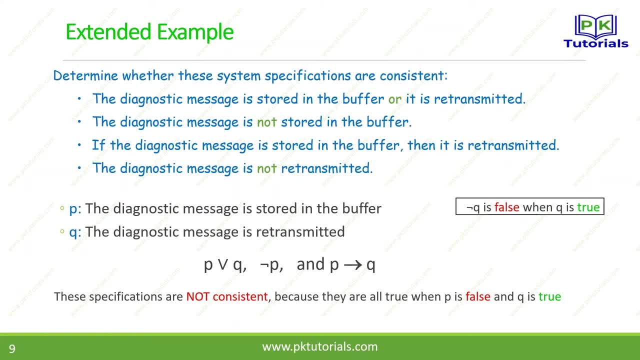 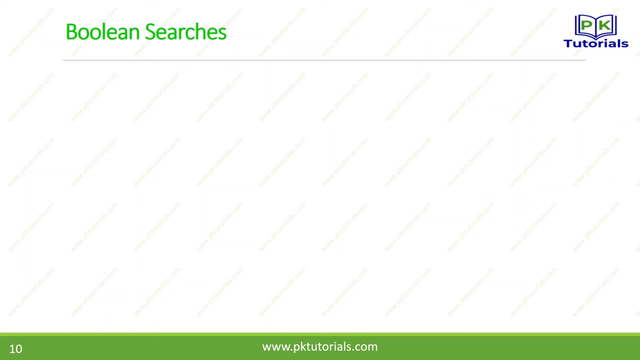 so these specifications are not consistent because they are all true when P is false and Q is true. if Q is true and P is false, then they are all true. so they are not consistent. now let's check the Boolean searches. in Boolean searches, how do we look at the logical propositions? 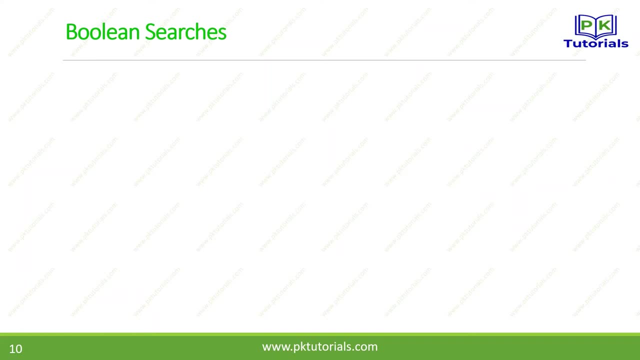 how do we look at the applications? how do we apply them? so logical connectives are used in indexes and web pages, the web pages of the website and the indexing of the pages, like Google does indexing. so when we look at the Boolean searches, logical connectives can be used. 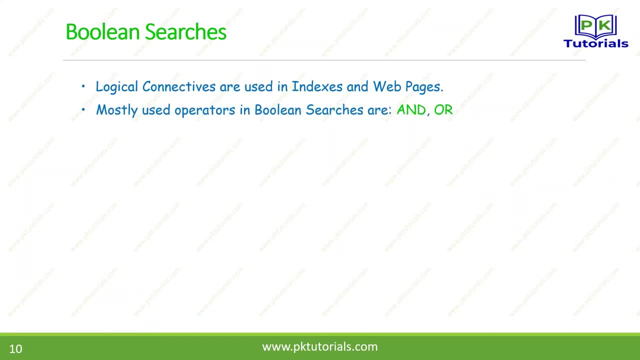 and mostly used operators in Boolean searches are and or are, and or are. we mostly use the ones with negation or the ones with not are very less used. let's check an example. if you go to Google search engine, for example, you search a sentence: I need job in Islamabad or Lahore. 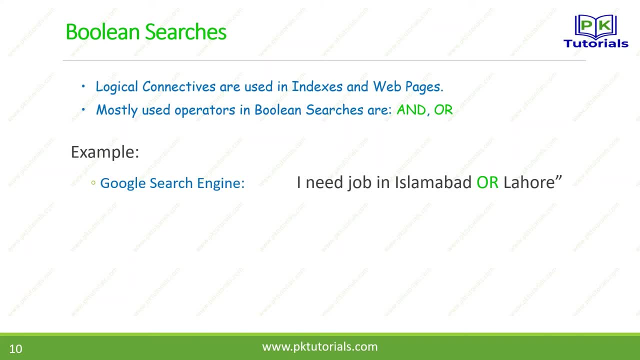 now what does Google do? it says that the R in this sentence is a logical connective and in that both options means you need the job in Islamabad or Lahore. so this R can be expressed through the logical connective to find the pages that deal with. 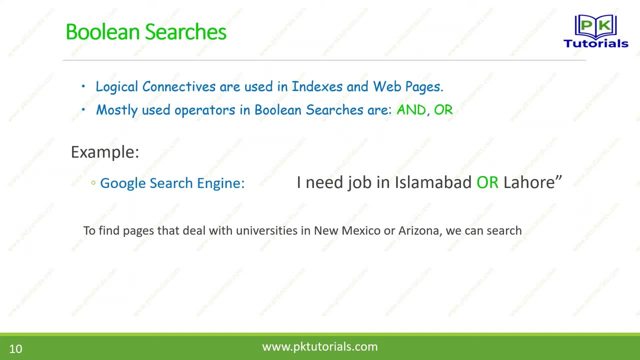 universities in New Mexico or Arizona. we can search similarly. if we search in Google search, we find the pages where the pages are found, the pages that deal with New Mexico or Arizona University. so how do we search New and Mexico? now see New and Mexico or Arizona. 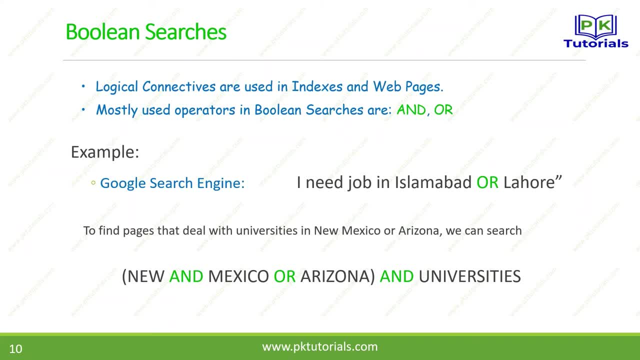 we put it in the bracket and, and universities. so this and, and are these are the logical operatives that we can use in Boolean searches. see, New Mexico is the same name, but if you write New Mexico directly and don't put the end in both, so this New. 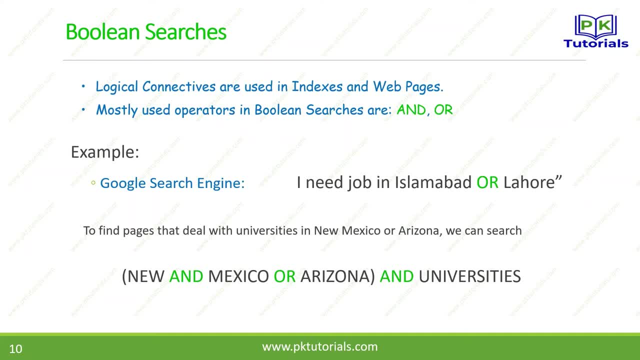 is different, like New Document, New Folder, New File, New Page, different New where it will be used. so it will search all the pages. we will put it in the result. but when you put the operator with it, and New Mexico, so where these two, New Mexico will come to the same place. 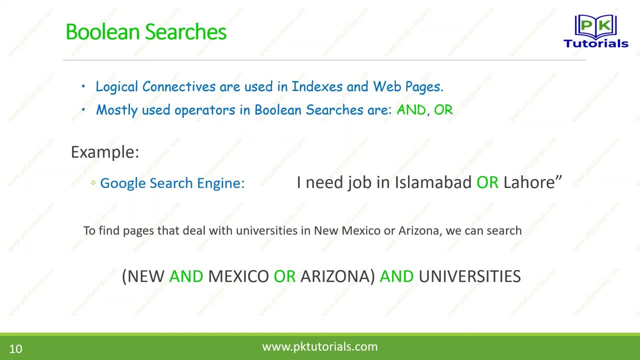 so we will search both of them similarly and Arizona and New Mexico and Arizona, one of these two- and University now see in University, we put it in the end with the bracket: both means wherever the University is in Arizona or New Mexico. so we will search all those universities. 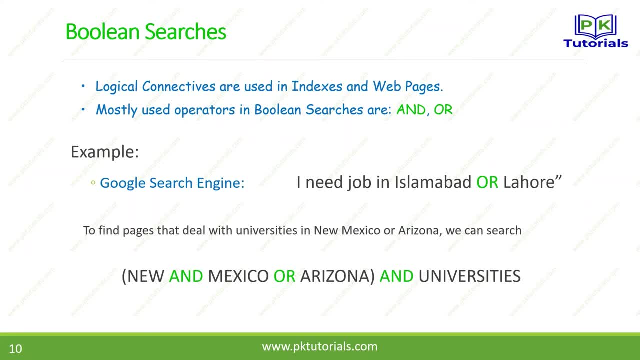 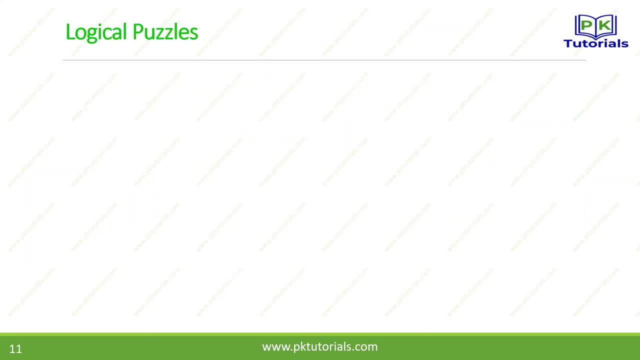 their pages. all of them. we will return to you in Google. so these are the examples of Boolean searches. where we logical connect, we can use the prepositional preposition. we can use it logical puzzle. third application: we will see how we can solve the logical puzzle. 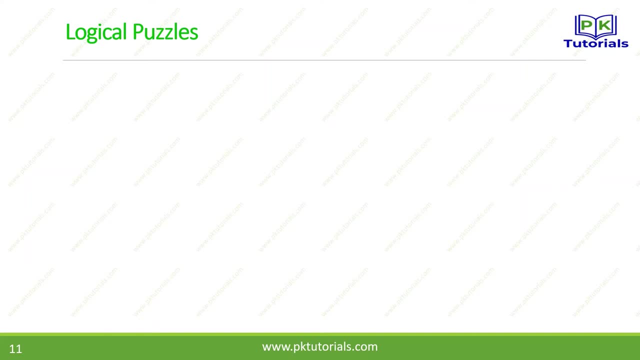 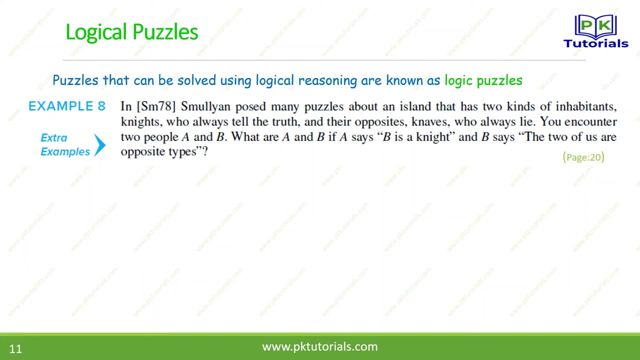 so puzzles that can be solved using logical reasoning are known as logic puzzles. which we can solve with logical reasoning, we call that puzzle logic puzzle. let's see an example. example is on page 20 of the book SM 78. its reference is in Somalian post. 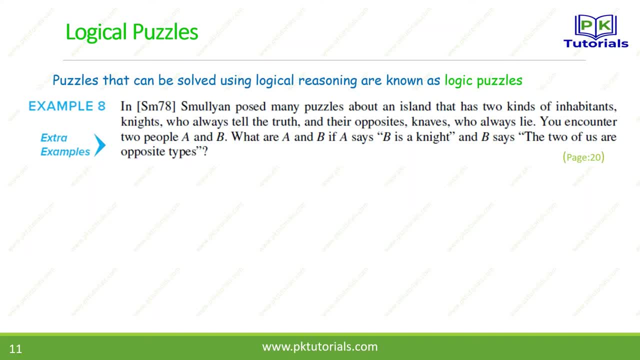 many puzzles about an island that has two kinds of inhabitants. inhabitants means people who live in an island. there are two types of people: Knights, who always tell the truth. note: Knights always speak the truth and they are opposite. Nau always lie. They always lie. they always tell lies. 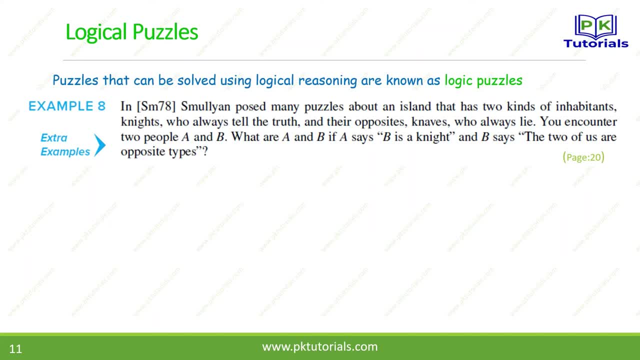 that is, there are two types of tribes. One is Knights and the other is Nau. Knights always tell the truth, while Nevs always tell lies. that is, you encounter two people, A and B. so you meet two people in an island. one is named A and the other is named B. 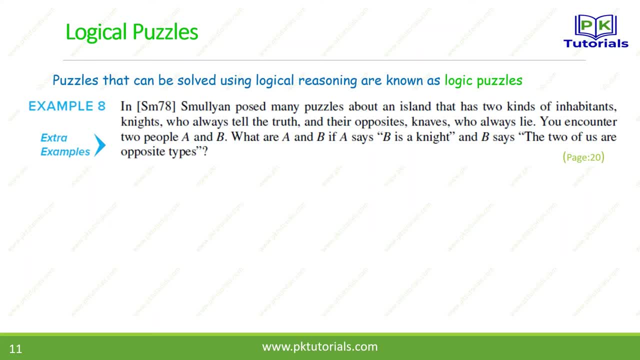 So what are A and B? if A says so, A and B, you have to find out that A is a knight or a knave and, similarly, B is a knight or a knave. The two people you have met, A. A has told you that B is a knight. 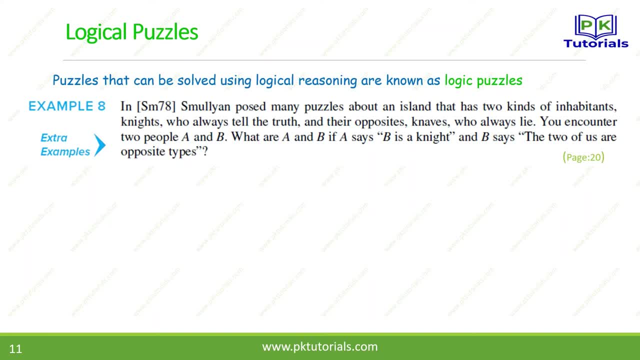 And B has said that the two of us are opposite types. So we have to logically prove that we have to solve this puzzle- that A and B are knights or knaves. So let's suppose P- A is a knight, We suppose that P is a knight, and suppose Q- B is a knight and B has a knight. 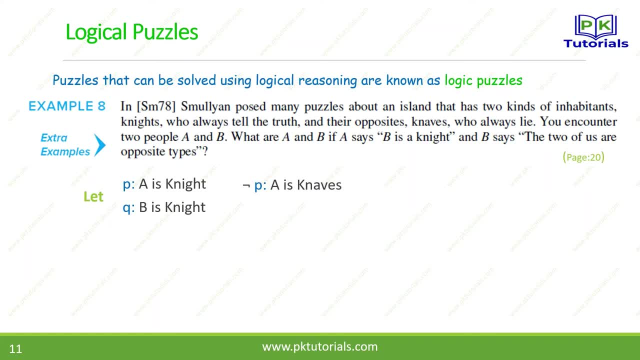 Similarly, N says that P is a knight and B has a knight. So the negation of P if A is a knight, if A is a knight, if P is a knave, then we denote it with the negation of P. 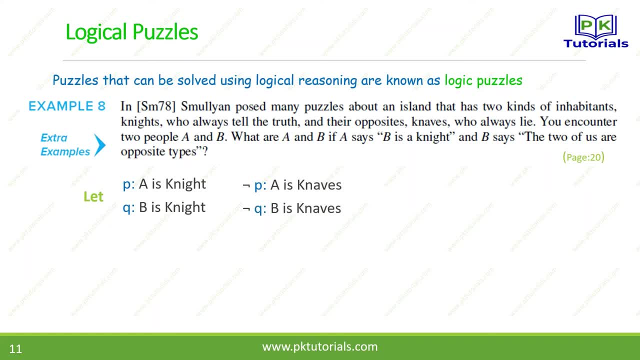 And similarly the negation of Q means that P is a knave. And in the above question two conditions have been given. The condition is that A says that B is a knight, A says that B is a knight And B says that B is a knight. 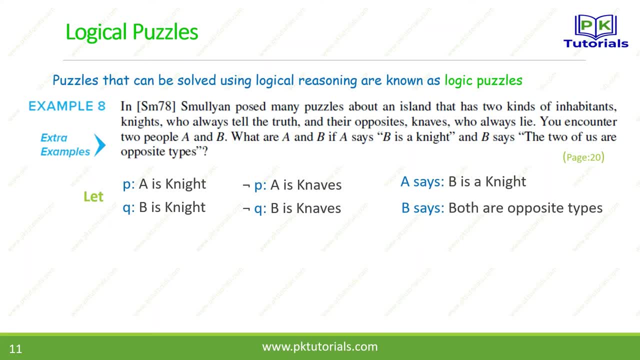 Both are opposite types. Now, according to these conditions- A and B- we have to solve this puzzle. How Now, since there are two, we have four available cases, Because P and Q, each one has a true and false value. 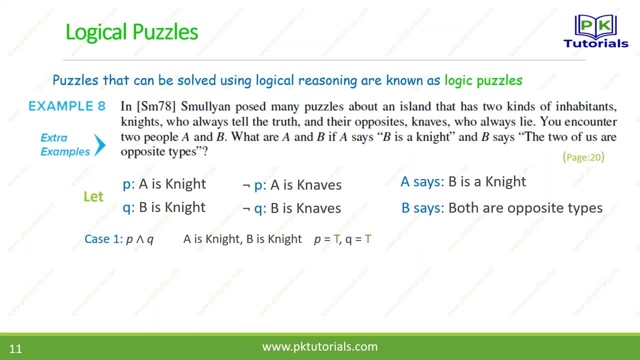 So we have two and two, four cases. So let's see the first case: A is a knight, B is a knight, Meaning P, Conjunction Q, P and Q, That both of us have a knight. 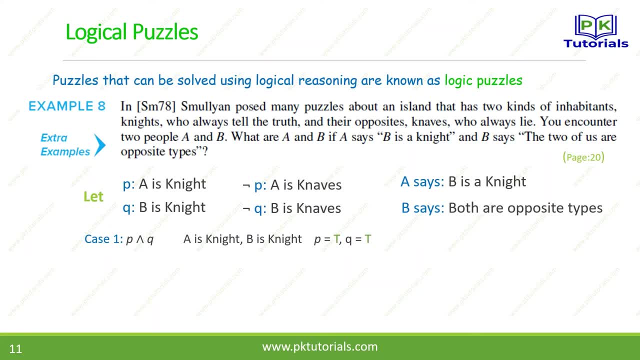 If P, then P is also true and Q is also true. So which case is this? P and Q? These are valid. Now let's see if A is a knight And A says that B is a knight, Because if A is a knight, then he always speaks the truth. 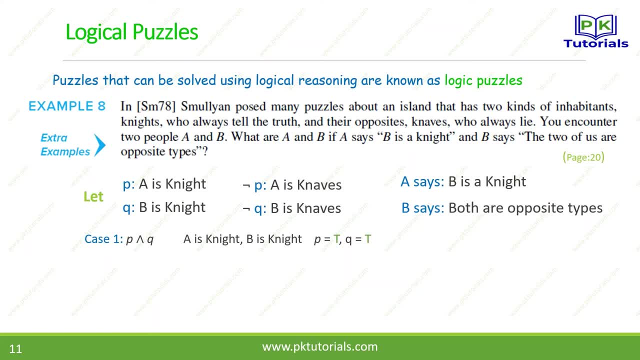 So B is also a knight. So B is a knight. So first A is correct, But B is a knight. Now the second is that if B is also a knight, then the knight also always speaks the truth. 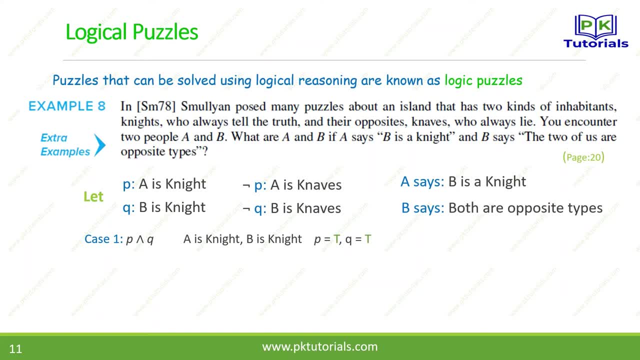 But B said that both of us are opposite types. So this means that B has lied. Our knight never lies. So it means that the second condition is not satisfied. So it means it is satisfied. So it means it is not a valid case. 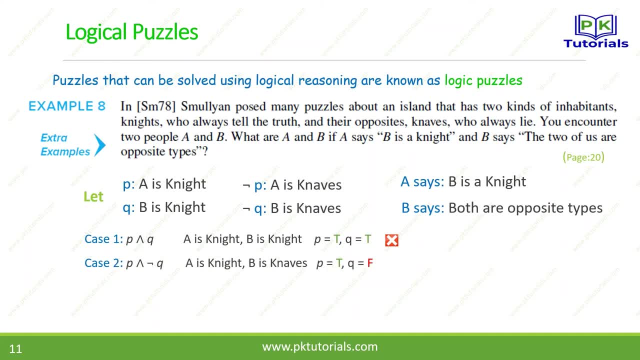 So in the second case we see that A is a knight and B is a knight. One is a knight and the other is a knight. Meaning: P and negation of Q. So P is true and Q is false. Meaning: negation of Q. 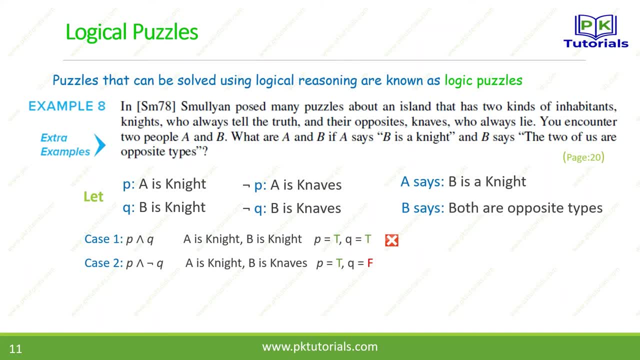 Let's see this Now. let's see: if A is a knight, So A is a knight, and A said that B is a knight Because the knight does not lie, then B is a knight, But in this case we have B is the news. 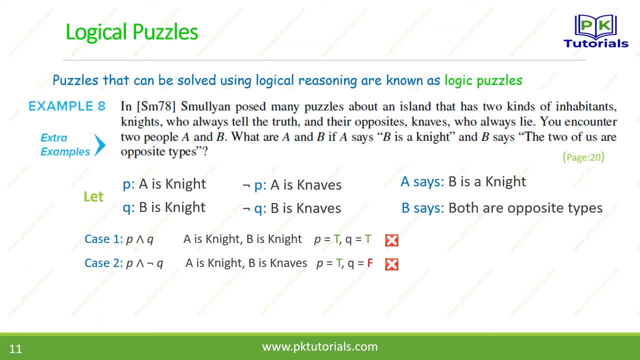 B is the news. So this is invalid and we cannot take this. So we have case 3.. Negation of P Meaning A is news and B is the night. Negation of P and Q. So P is false and Q is true. 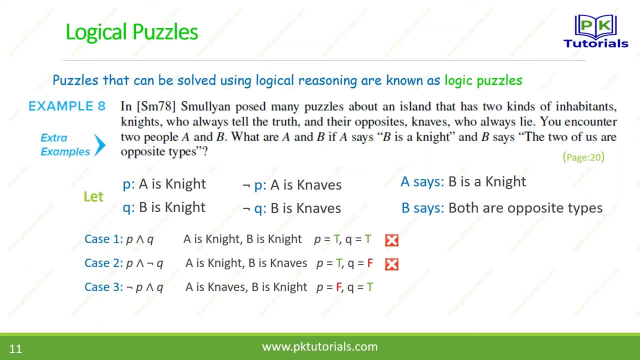 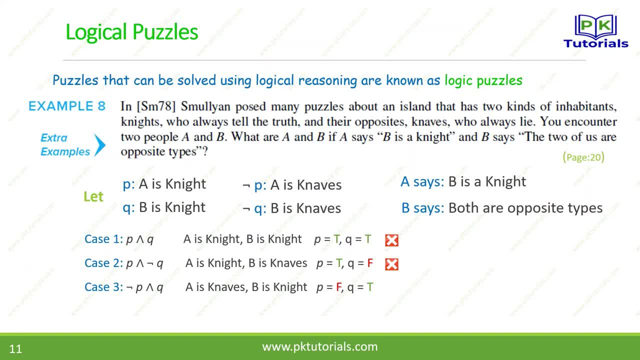 B is night. Okay, Now A: if it is night, it means that he is lying. If he is lying, then B will not be night. it will be night, But B is night. So this condition, the first condition, 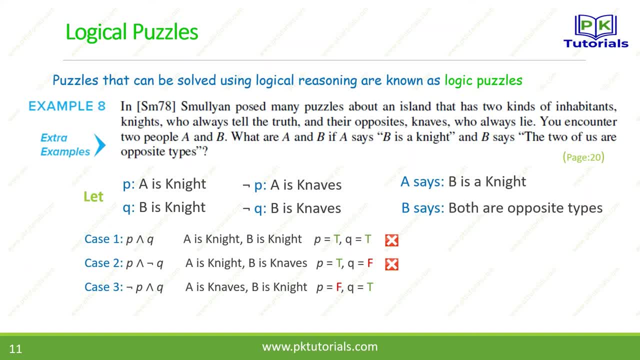 is false. The second is true because both are opposite types, Because one is night, one is night, The second sustains. but the first condition is irrelevant, It is wrong, It is invalid. So this also does not fulfill our case. 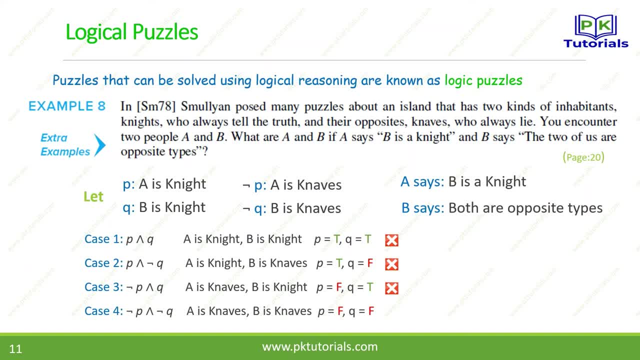 The fourth case is negation of P and negation of Q, Meaning A is also night and B is also night, So P is also false, Q is also false. Let's see now: A is night Means: 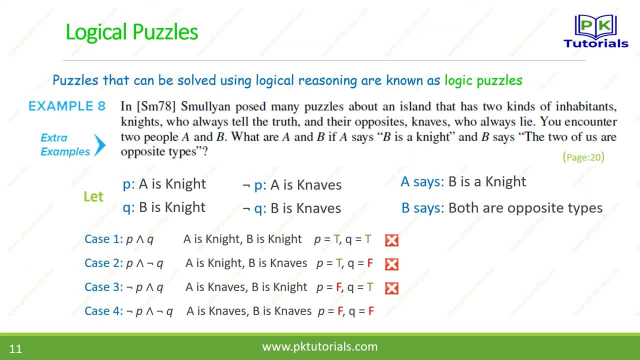 A said B is night Meaning. he lied Because nights always lie. So B is not night, it is night Meaning he lied. So the first condition is true Meaning it is valid. Okay, B is night. 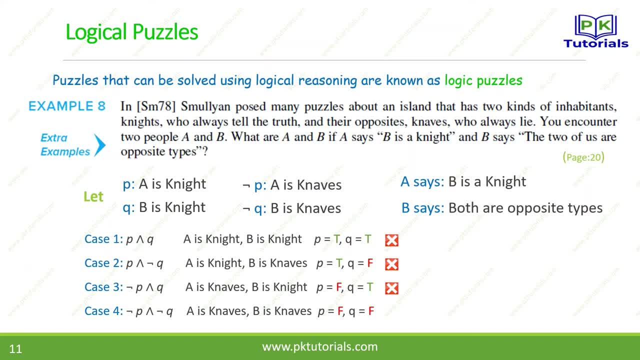 B said that both of us are opposite types Meaning we are opposite types Meaning we are opposite Meaning we are night and the other is night. So he lied Because we are night So we always lie. 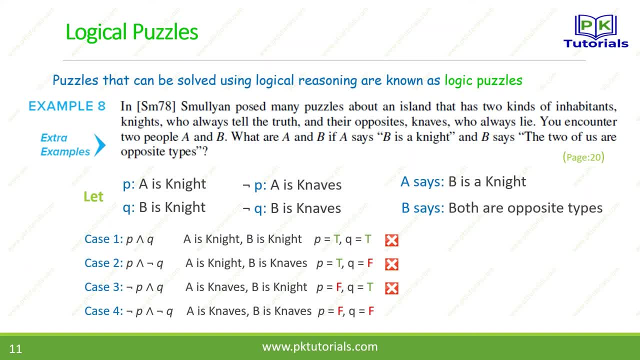 We are not opposite types, Meaning we are the same type. So both conditions we have valid in this. So that's the solution of this logical puzzle, Because both are naives. Let's repeat this a little bit.